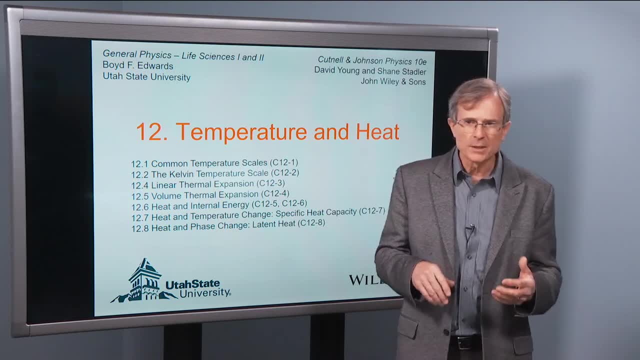 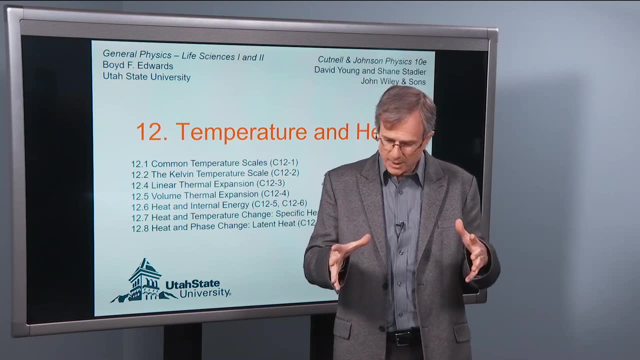 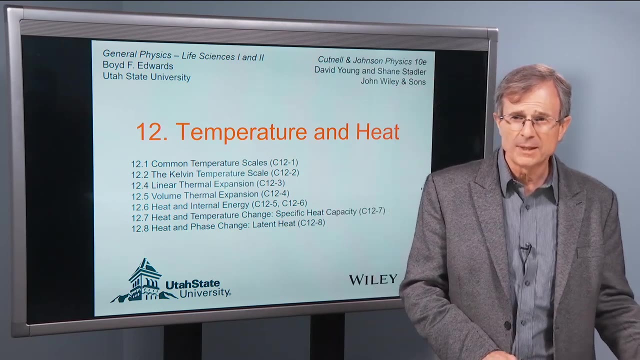 In this chapter we'll talk about temperature scales: the Kelvin scale, the Celsius scale, Fahrenheit scale, linear thermal expansion- If you heat something, it expands. We'll talk about internal energy and temperature changes, specific heat capacity and latent heat. 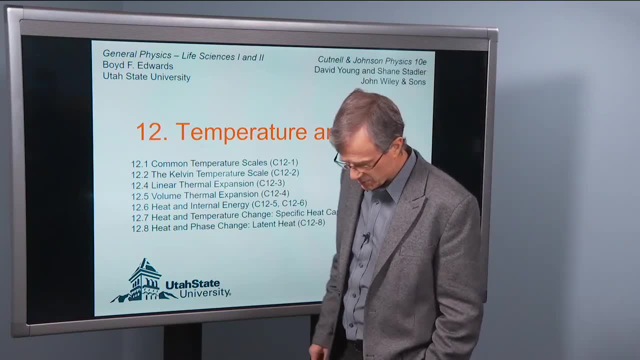 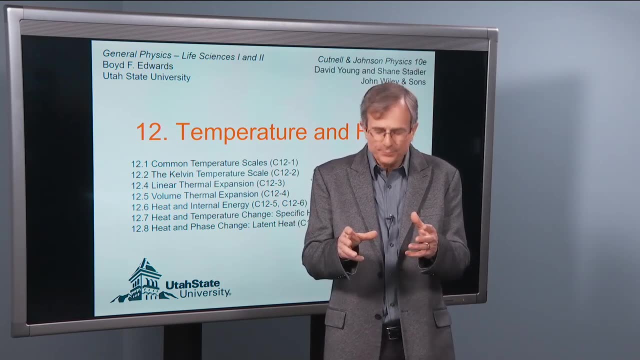 That's the heat associated with the phase change. So if you- we were just trying to thaw out some shrimp the other day and you take this frozen shrimp and put it in water and then you mix it around a little bit to thaw the shrimp out, 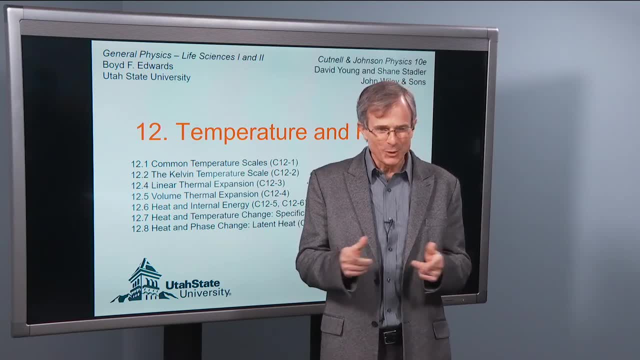 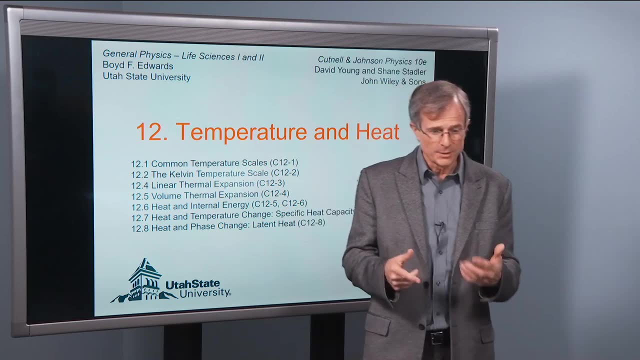 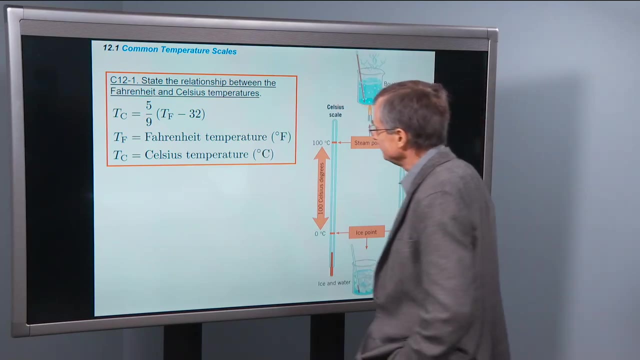 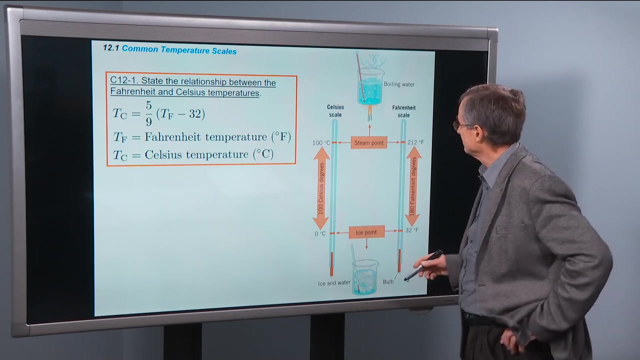 and the water gets cold very, very fast. There's a lot of heat associated with changing the state from frozen or solid to unfrozen. That's called latent heat. Okay, so temperature scales. Here is the two most commonly used temperature scales. 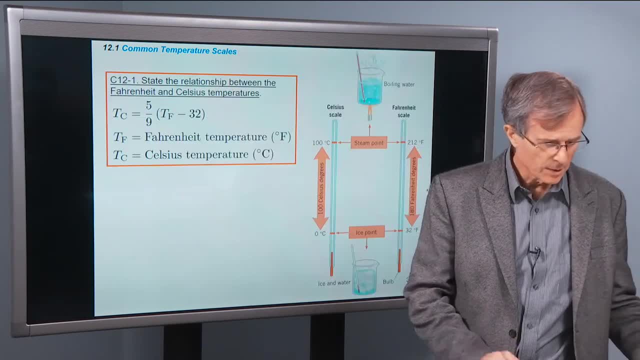 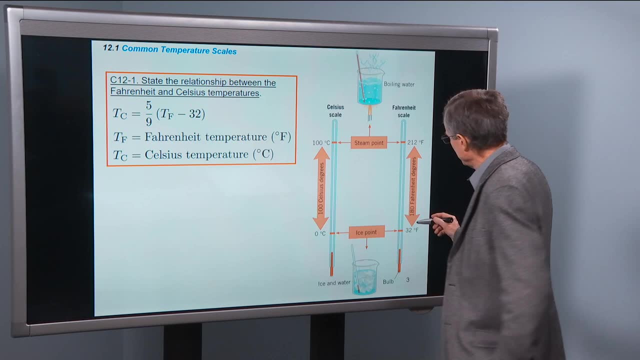 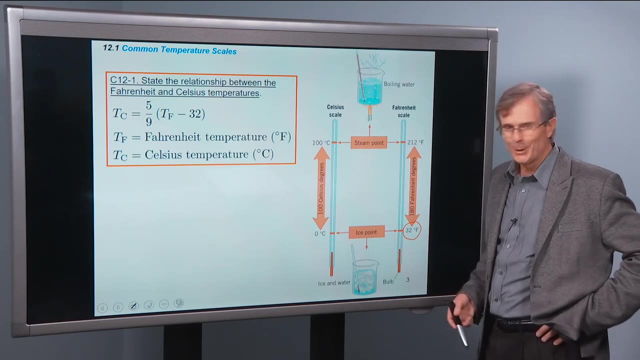 The Fahrenheit scale that we use every day. how many degrees Fahrenheit, et cetera, et cetera. And the ice point, the freezing point, is at 32 degrees Fahrenheit, as you might well remember, because below 32 is below freezing. 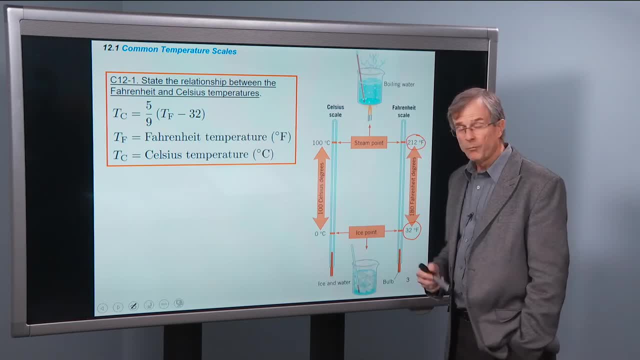 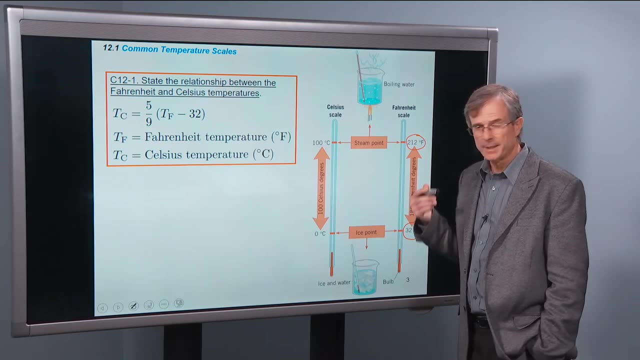 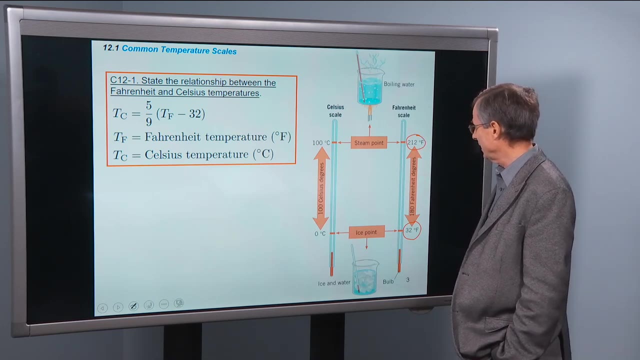 You might also remember the boiling point of water at atmospheric pressure. standard temperature and pressure is 212 degrees Fahrenheit. Well, that's kind of an embarrassing uh temperature scale. I don't know who invented it, I guess a guy named Fahrenheit. 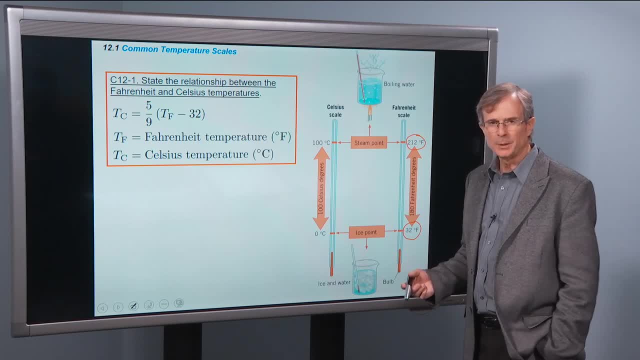 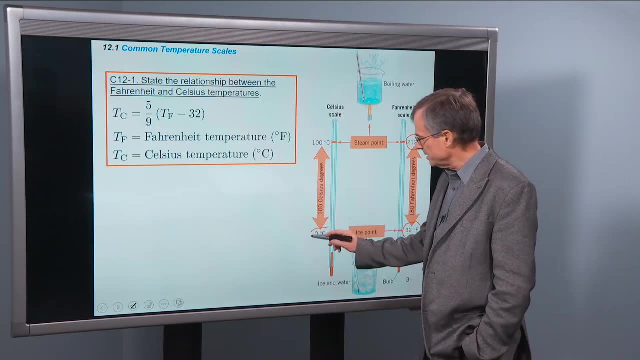 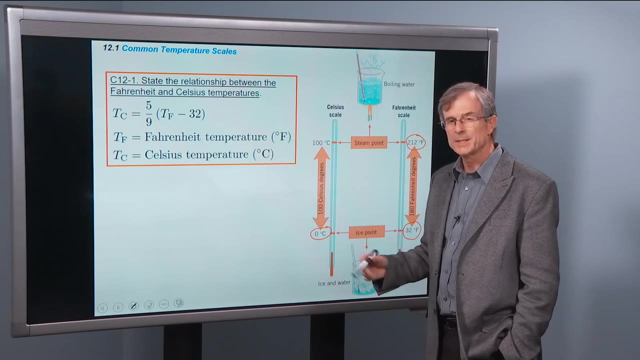 Um, a more useful scale, a little bit more tied to our natural phenomena in the world, is called the Celsius scale, where the ice point is zero degrees. So when the temperature on the Celsius scale is below zero, that's below freezing. 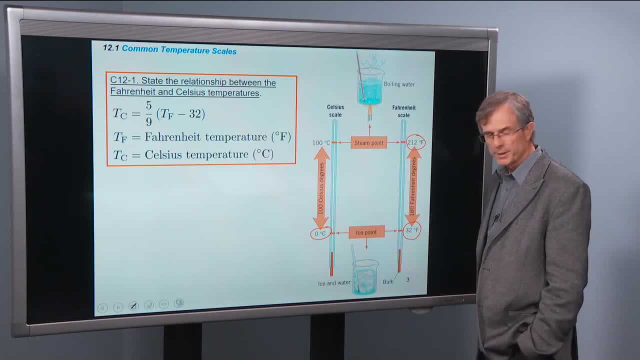 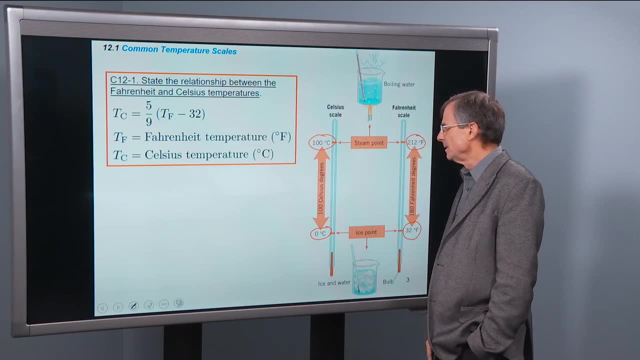 The same as saying that the temperature is below 32 degrees Fahrenheit And 100 degrees is the um, the high end, the boiling point or the steam point where you can convert water into steam, And there's a 100 degree Celsius degree difference. 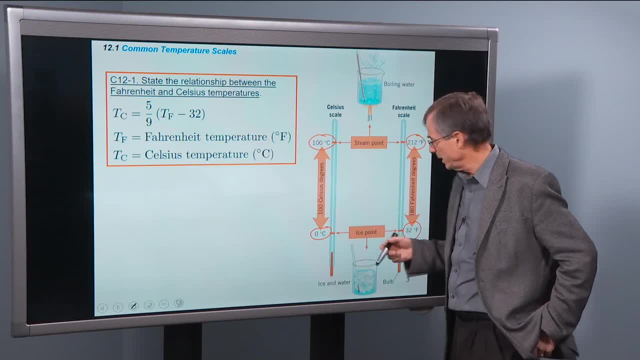 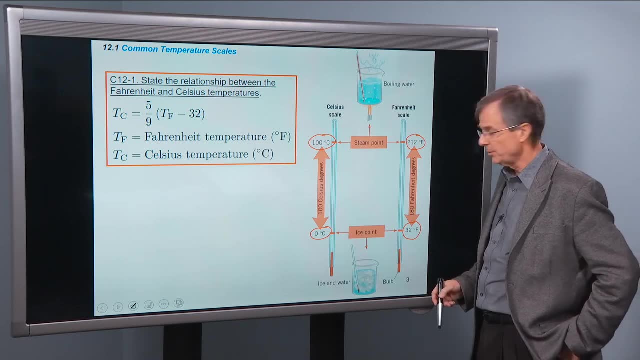 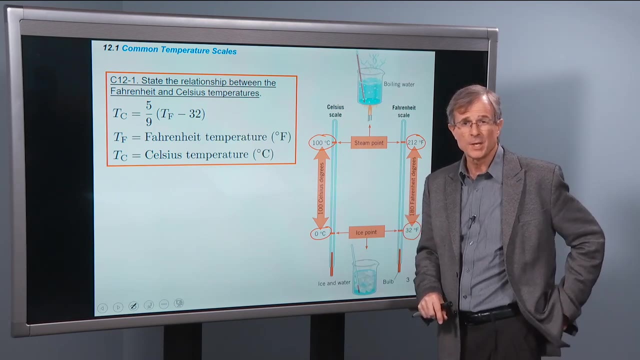 between the ice point and the steam point, whereas between 32 and 212, if you take 212 minus 32, you get 180 Fahrenheit degree steps. So the Fahrenheit step is a smaller step. uh, changing things By one degree Celsius, you change it quite a bit. 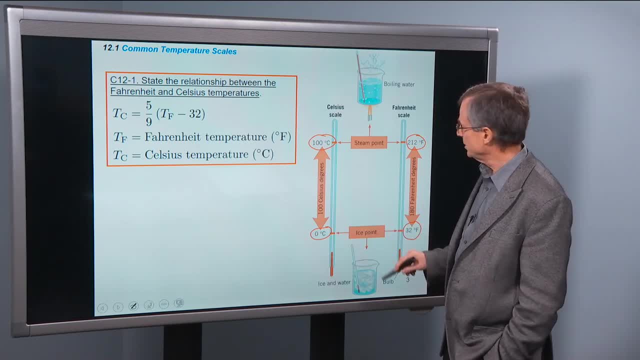 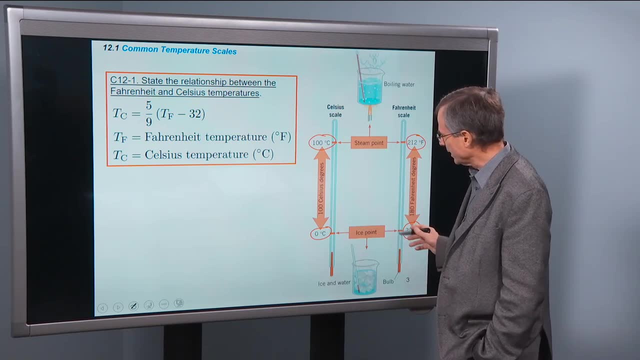 How do you relate the two? And the answer is uh, given this information, which I think uh you've all maybe seen before, um, you can figure out how to convert a temperature in Fahrenheit to a temperature in Celsius. And first of all, 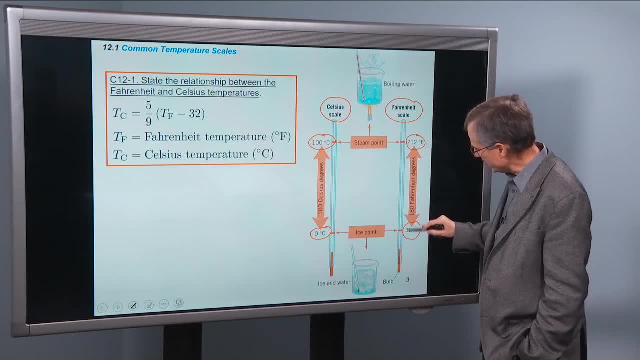 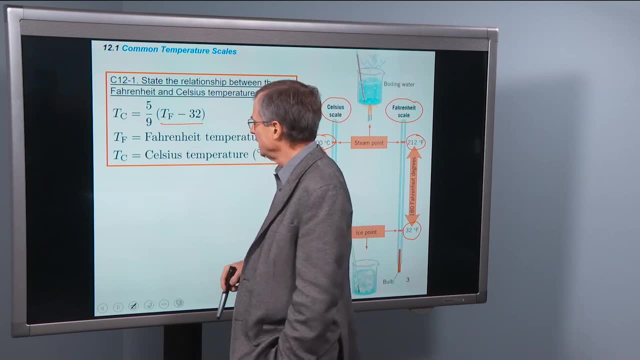 what you want to do in order to get it right is you want to subtract that 32 off, uh, and that's what you do- The temperature in Fahrenheit minus 32, and then you want to realize that um a a change in. 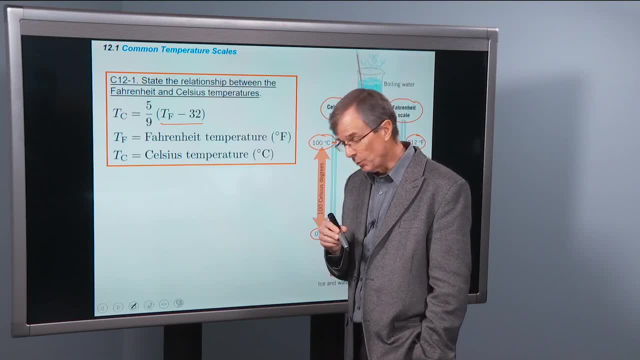 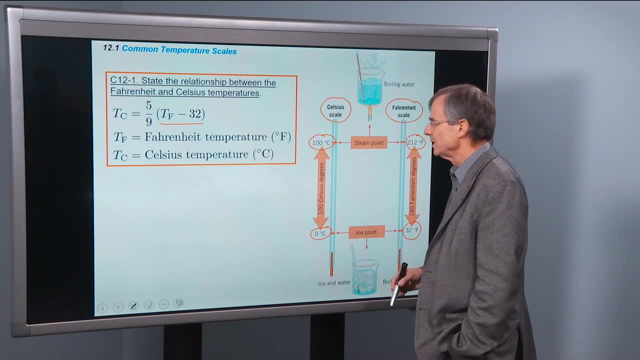 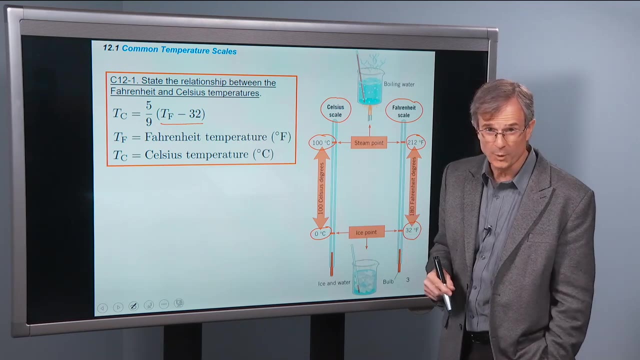 uh. one degree Celsius is a less of a chan- is is more of a change than um. so for any given uh temperature change in Fahrenheit, the corresponding change in Celsius is going to be less, because the degree in Celsius is more is more. 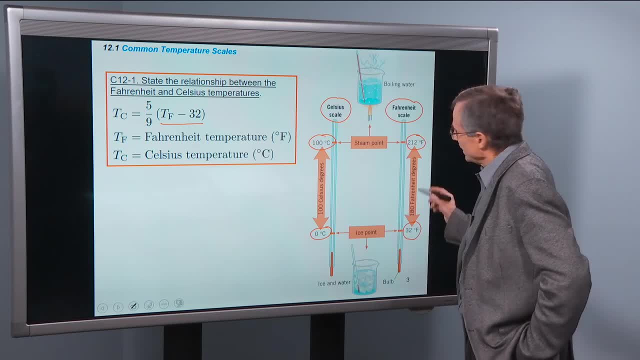 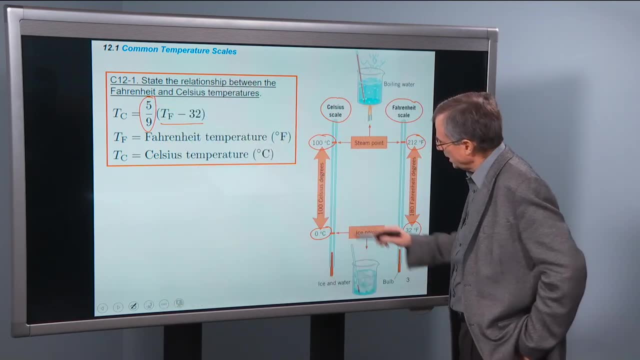 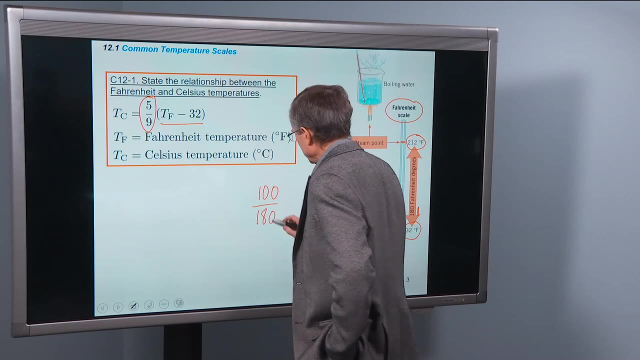 So I don't know if that made any sense or whatever, but um the conversion factor here, five-ninths. that comes from the ratio of 100 degrees to 180.. So 100 divided by 180, well, if you divide numerator and denominator by 10,. 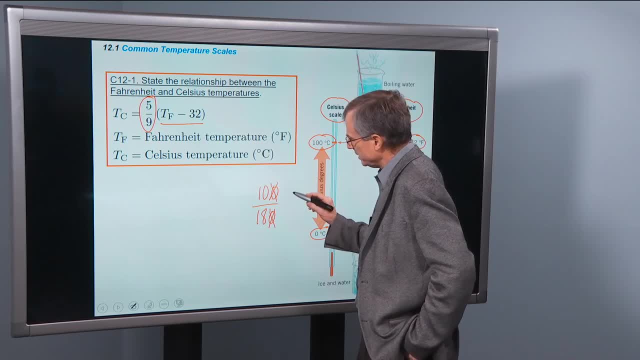 10, you get 10 over 18, and then divide each by 2, you get uh, 10 divided by 2 is 5,, 18 divided by 2 is 9.. So this is the uh, the ratio, uh. 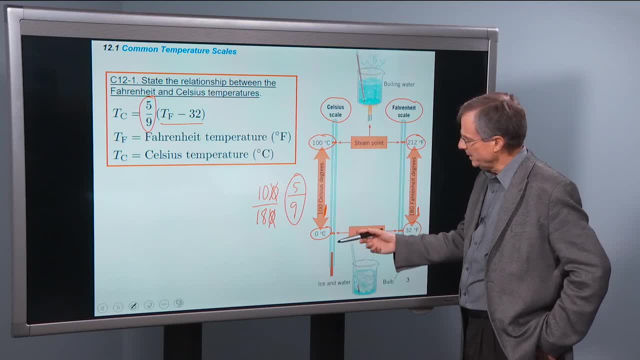 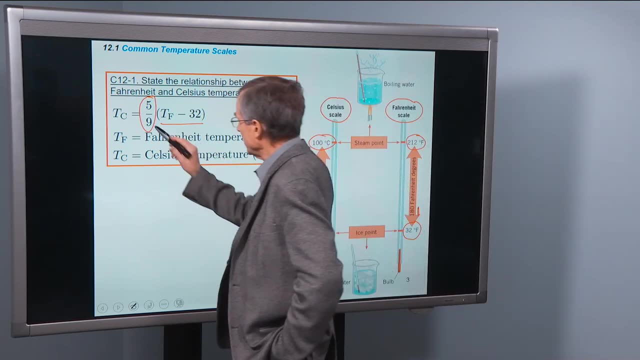 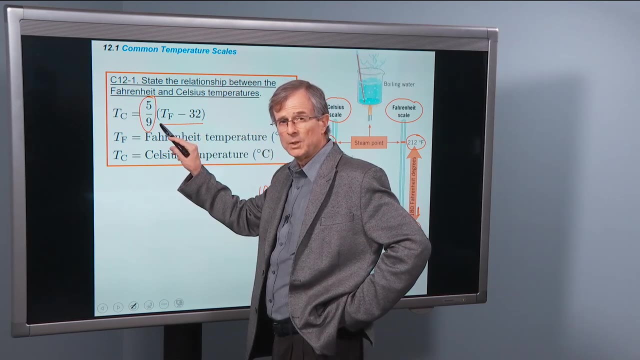 the ratio between the, the number of degrees between ice and steam for each of these two. So that's how this one comes out And we can double check to make sure it's right. If the temperature in Fahrenheit is 32, then 32 minus 32 is 0,. 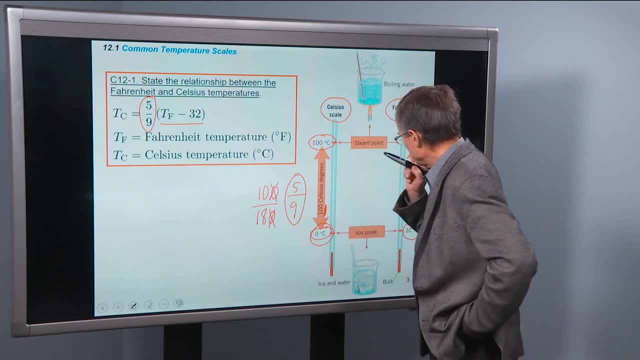 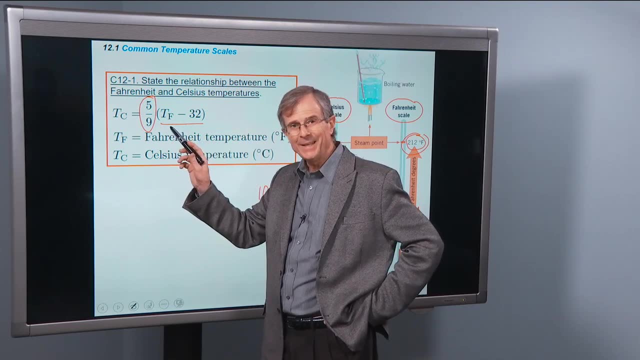 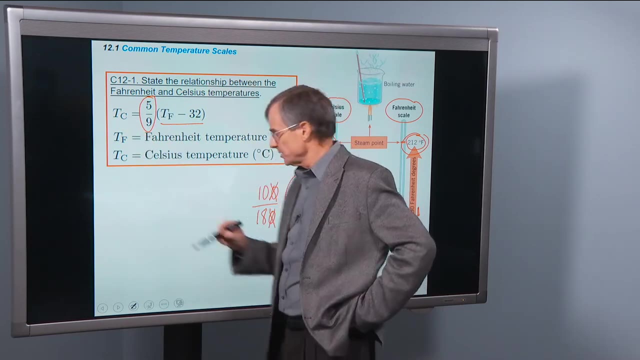 and the temperature in Celsius is 0.. If the temperature in Fahrenheit is 212, we put that in here- 212 minus 32 is 180, and five-ninths of 280,, as we just showed, is 100.. 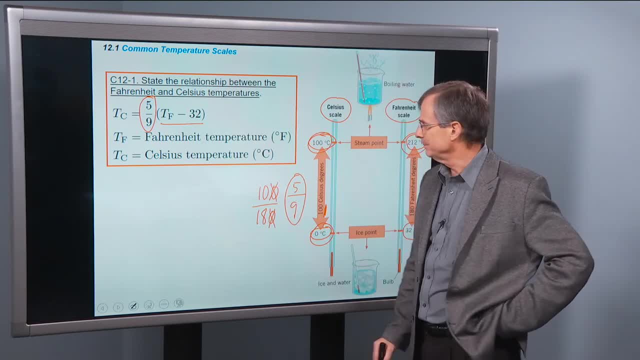 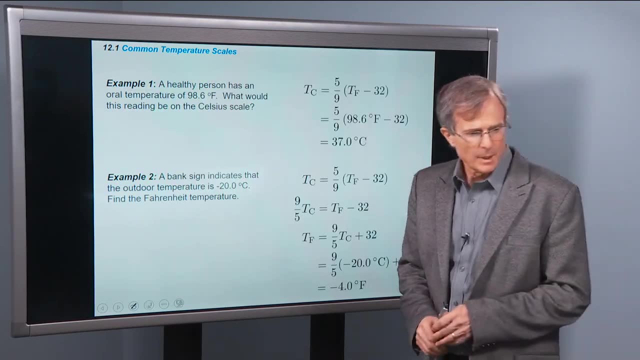 So that gives you this 100 degrees here. So five-ninths Tf minus 32.. No big deal. I think you've uh seen this before. Uh, just a couple of quick examples. A healthy person has an oral temperature of 98.6.. 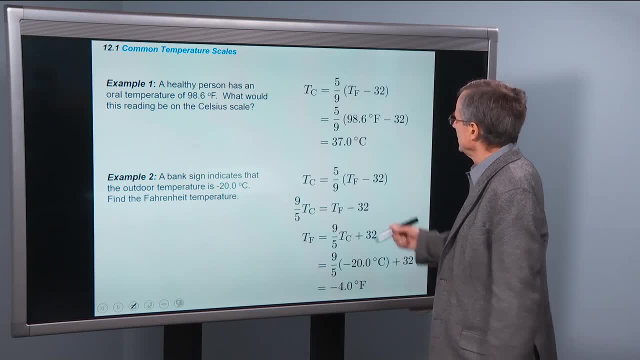 What would this reading be on the Celsius scale? Um plug it into the equation T, Fahrenheit is 98.6 minus 32, uh gives 37 degrees uh Celsius. This is a normal uh body temperature in Celsius. 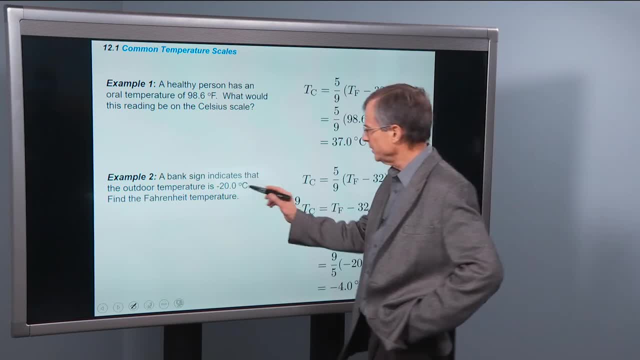 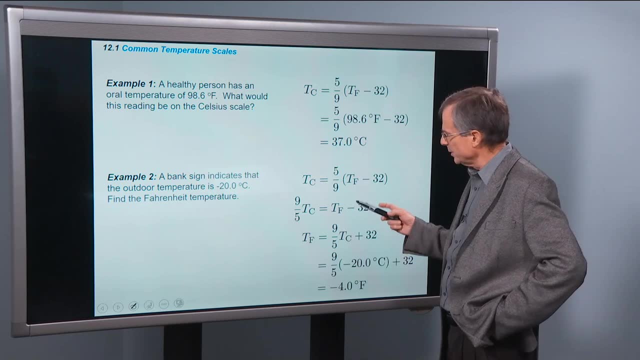 A bank sign indicates that the outdoor temperature is negative 20 degrees Celsius. Find that, uh? Fahrenheit temperature. Um, now for this one. we need to solve for the Fahrenheit temperature. So how do we do that? We can multiply both sides by 950. 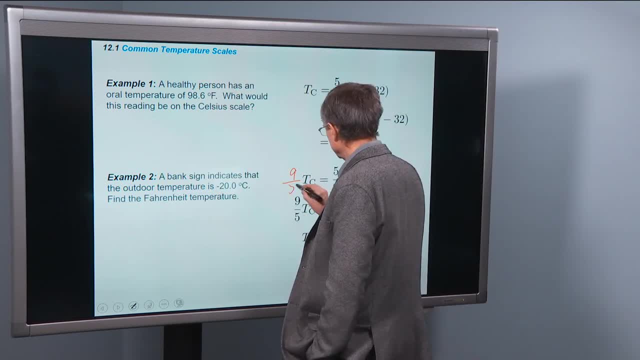 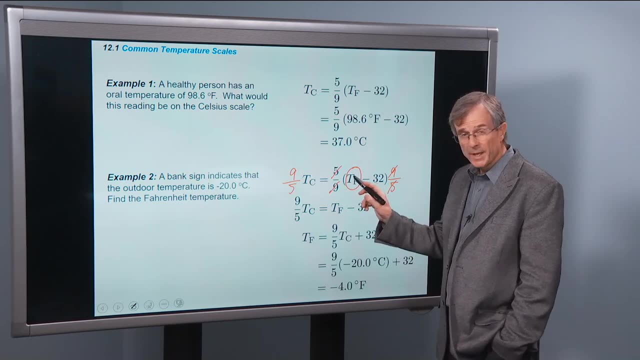 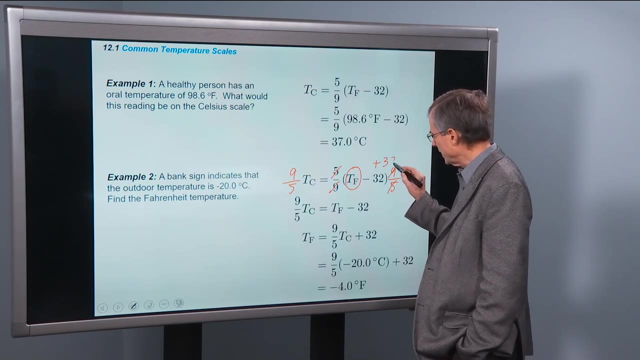 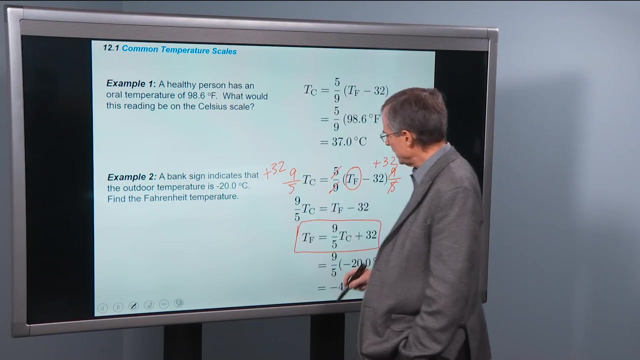 And this 5 cancels that 5.. This 9 cancels that 9.. So well, now we have Tf minus 32 equals nine-fifths Tc, And so we can add 32 to both sides and get that the temperature in Fahrenheit is nine-fifths Tc plus 32.. 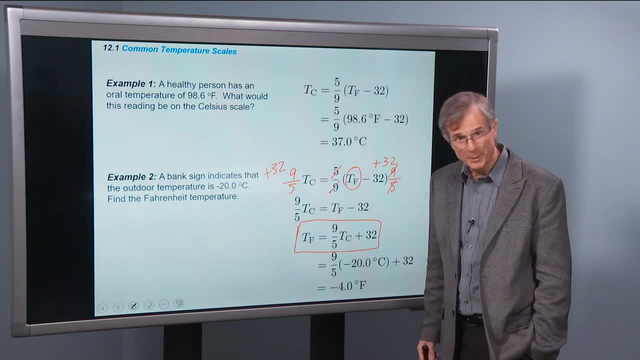 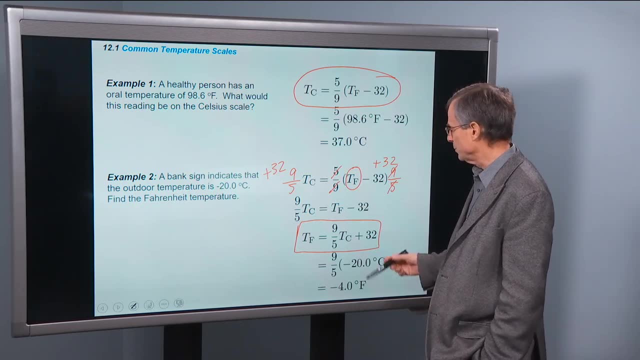 Now you can memorize this equation if you want, but I think it's dumb to memorize that equation I I like to keep the number of equations I need to memorize down to a bare minimum And then just do algebra. 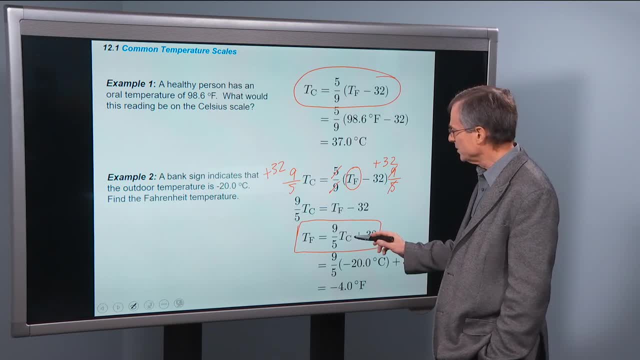 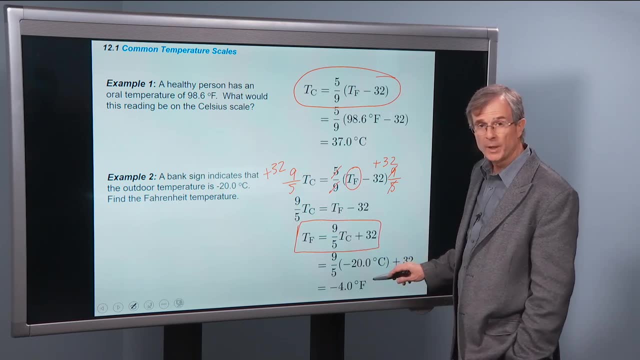 You can do this algebra, it's easy. So we've just uh shown that T Fahrenheit is nine-fifths Tc plus 32. We're putting in Tc as negative 20. And uh plug the numbers in. 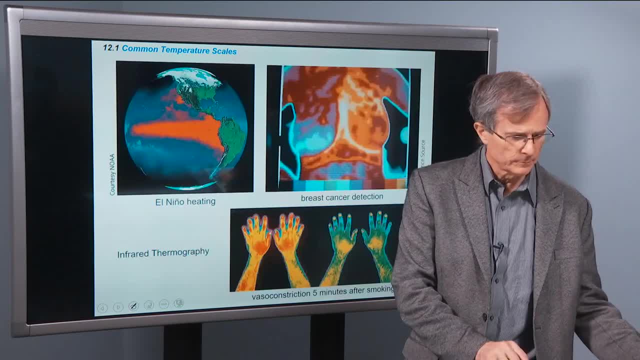 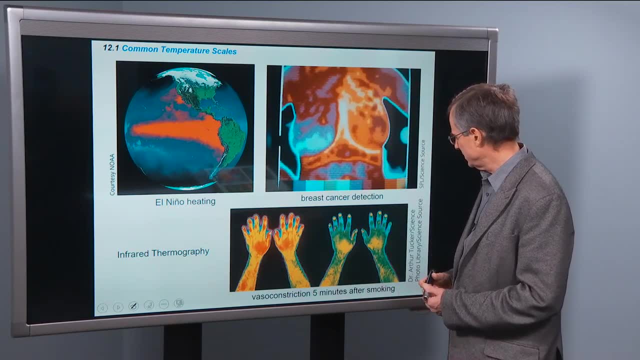 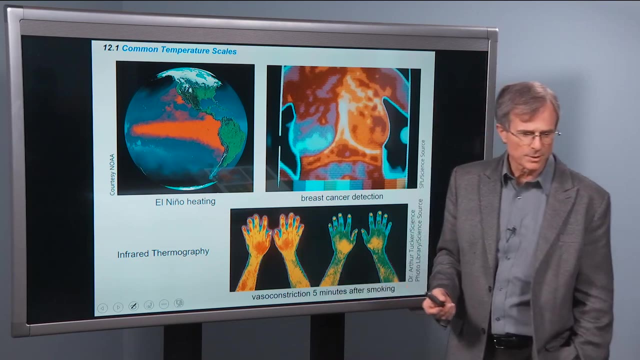 you get negative four degrees. Um temperature scales are. it's are valuable in thinking about uh vasoconstriction, Um. infrared um is used as a measure to to measure uh therm, uh temperatures. 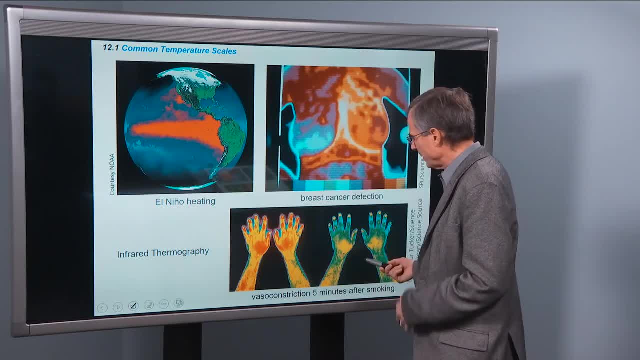 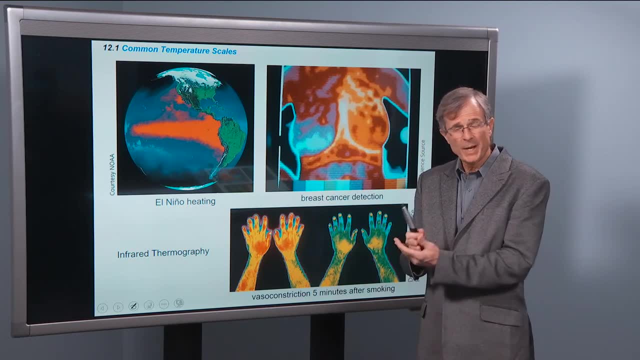 The temperature of of different body parts. um, this is a demonstration of how uh your your uh blood vessels constrict when you smoke, So your hands actually get colder. This is a demonstration of uh bre breast cancer.